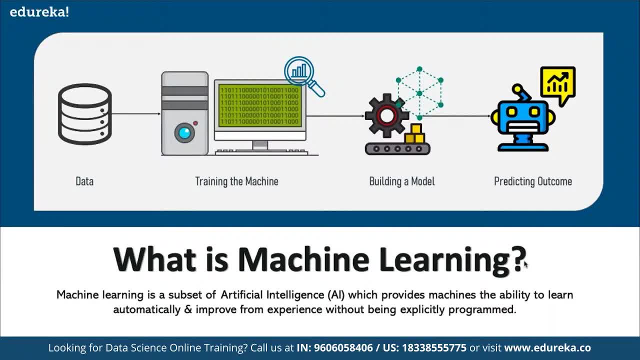 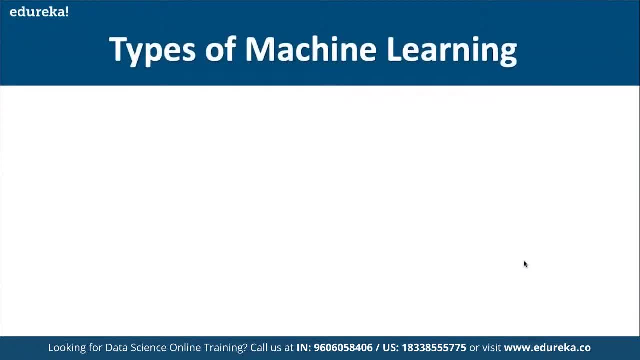 The egg. there goes a lot of processes, algorithms, and this is a factors to get the optimum results All right. so here, basically, We have three main types of wasly learning as well, where we have supervised, Unsupervised, and then we have reinforcement learning. so supervising- simple terms just trained me. 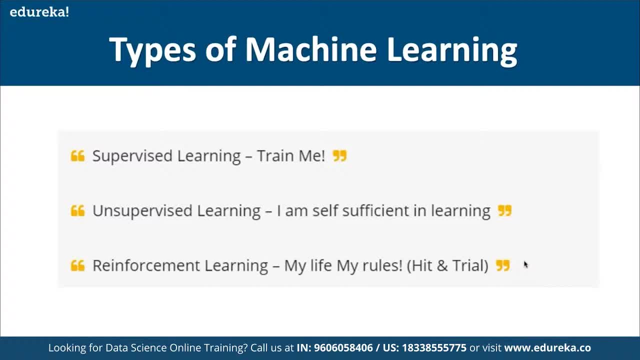 It was on a simple trading more. We have trained a model: the no-deal- It can work- and an unsupervised- only Is I'm sufficient vê Allow them to half, we're going to allow them to Have the access as well. So there is what. 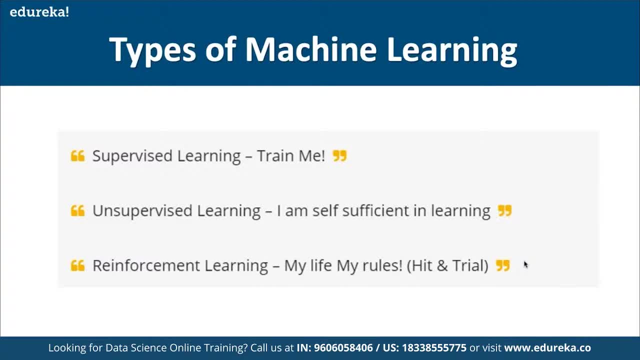 are going to define. so, based on their own understanding, they are going to work accordingly. that's how it's going to work. and then we are going to work on reinforcement learning. so reinforcement learning is simply learning on its own, based on the feedback we simply create. we 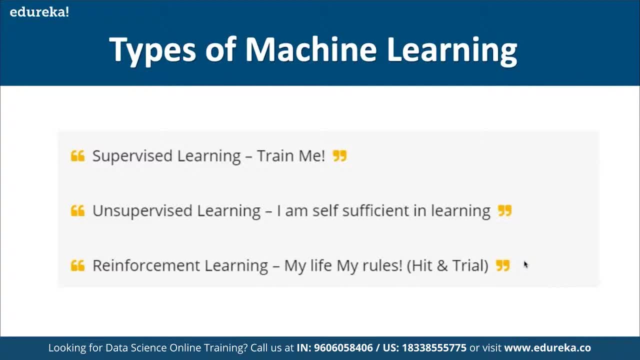 simply let the system know, okay, if they have done a good job or not and, based on that only, they simply try to get the best part of the possible output. that's how it works, all right, so supervisor searching. in supervised learning, we use multiple label data set to train the system and under 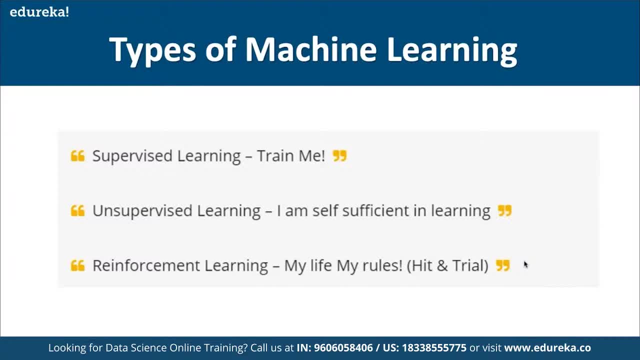 unsupervised learning. we use unlabeled data set, so the data is sometimes unlabeled or we can say uncategorized, and the machine makes the best, the best possible reference and predictions without any supervision. and then we have reinforcement learning. so reinforcement learning simply ensures: okay, we are simply going to create a system based on the feedback. 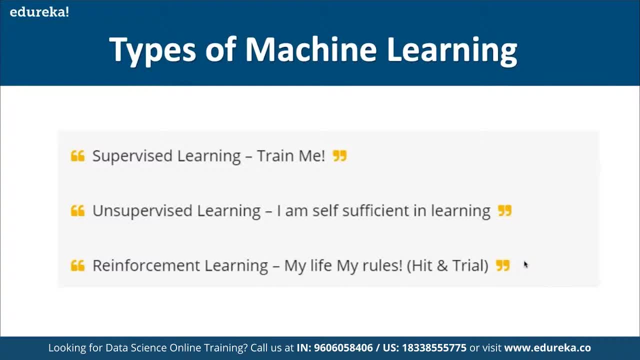 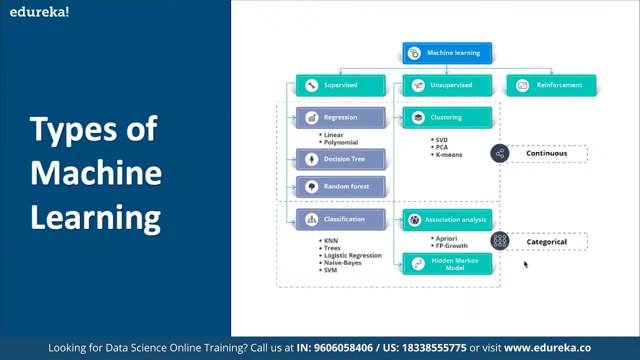 so the machine needs to establish a systematic pattern of approach and reinforcement learning here. so that's how we discuss again here we have supervised, again under supervised. we have multiple models, like we have regression decision tree. we have reinforcement models. we have different models currently available, whereas in under unsupervised we have multiple models, like we have clustering. we 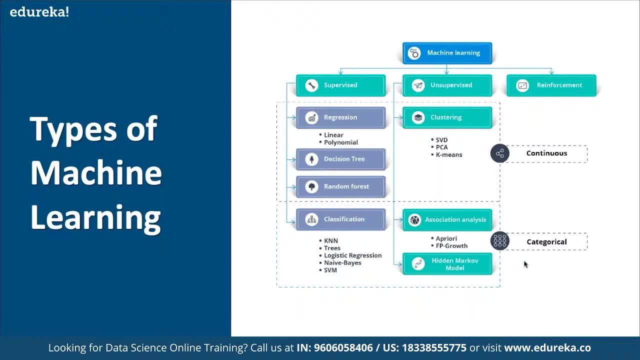 have association analysis, we have hidden markup model. so again, the knn trees, logistic regression, logistic regression, knife base, and we have. they all are types of classification where, if we talk about the upper theory, fv growth, k means pca, svd- they all are part of unsupervised and, again, reinforcement is simply based on. 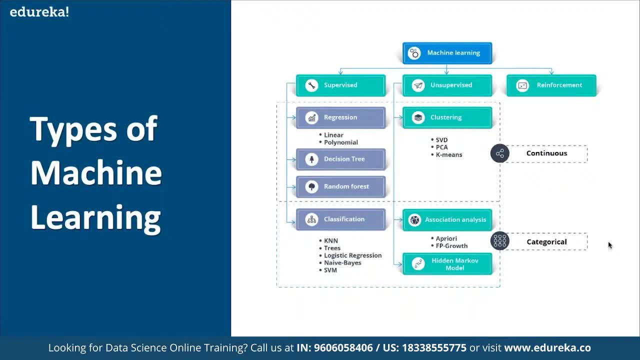 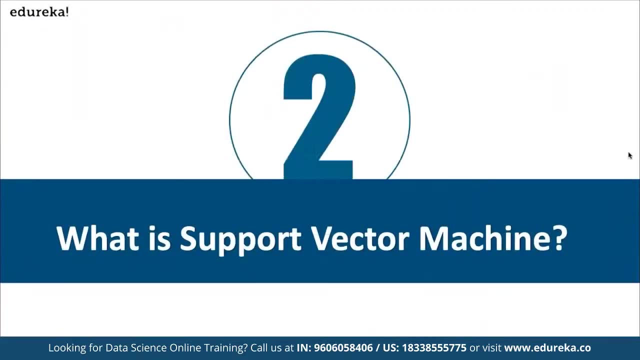 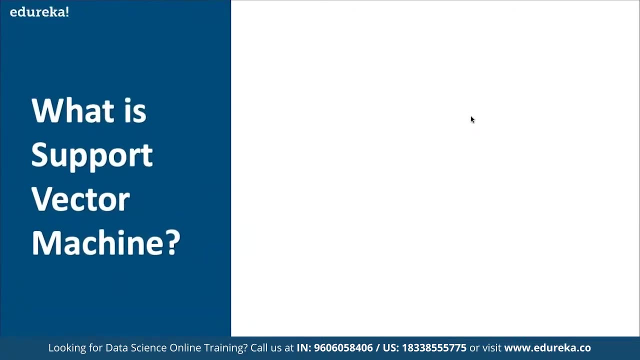 its own structure that we are going to discuss as we proceed further, step by step. all right, so now next is we are going to discuss on what exactly we mean by support vector machine. so a support vector machine was first introduced in the 19th 60s and later improvised in 1990s as well, and it has basically a supervised learning machine. 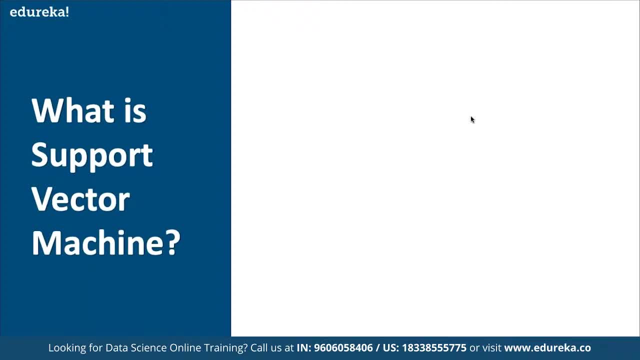 classification algorithm that has become extremely popular nowadays because of its- you can say- efficient results and especially for the complicated scenarios, it can deliver it for us as a part of support vector machine. as you can see again simply, there's like a discriminative classifier that is formally designed by a separative 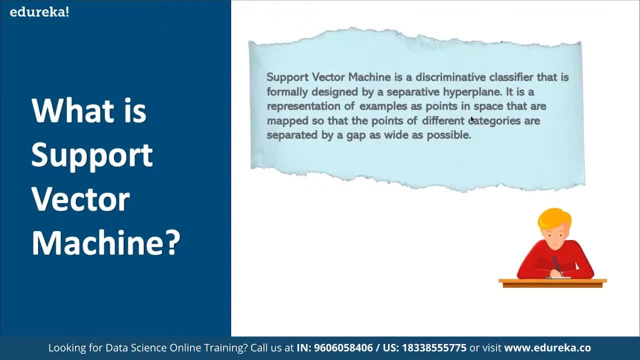 hyperplane itself, and svm is implemented in a slightly different way than the other machine learning algorithms, so it is capable of performing classification, regression and outline direction as well, and support vector machine is basically again simply designed by the separative hyperplane set as we discussed. so basically, here we can have multiple data. 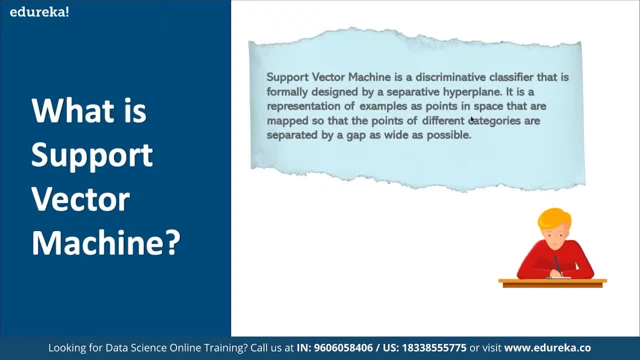 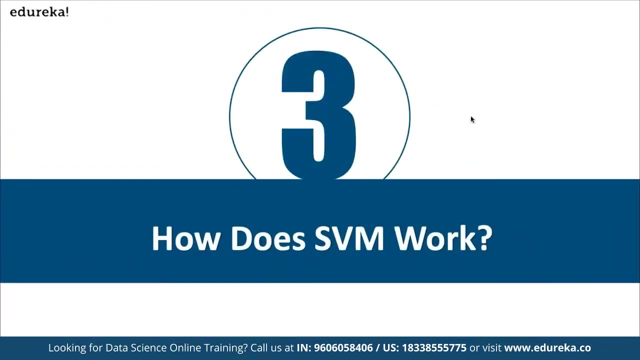 pointers that can be mapped, so that the points of different categories are going to be separated by a gap, and in addition, so basically, svm can also perform non-linear classification. so we'll be talking more about the sub, how exactly support vector machine works, as we proceed further. 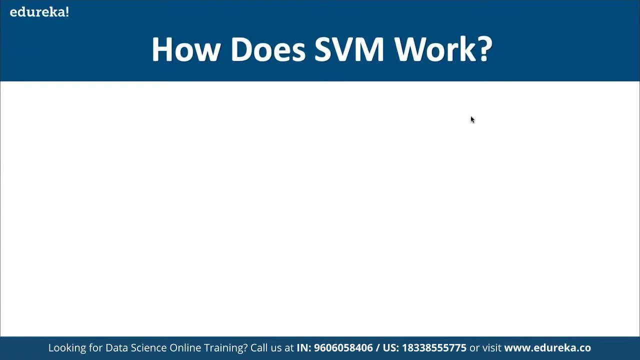 but there are multiple advantages of using svm as well. for example, it is effective in high dimensional spaces, it is effective in cases where the number of dimensions in greater is greater than the number of samples, and it is okay. it simply uses a subset of trading points in decision function. 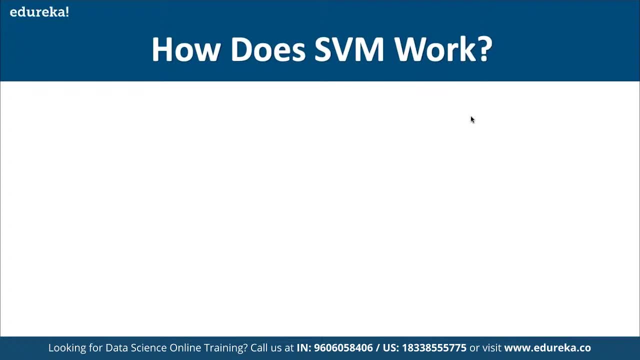 that makes it memory efficient and it has different kernel functions that can be specified for decision function. that also makes it versatile. and the same way we also have multiple- we can say downside or we can say disadvantages of using svm as well. so the number of features is much larger. 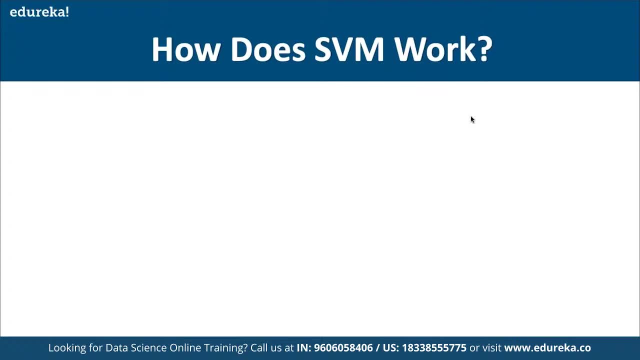 than the number of samples. then we can simply avoid overfitting and choosing kernel functions. and again, recognizing them is crucial, and svm did not directly provide any of these features, but it does provide a number of features that we can use in order to make sure that we are able to use these features in the right way. so, for example, if we want to use 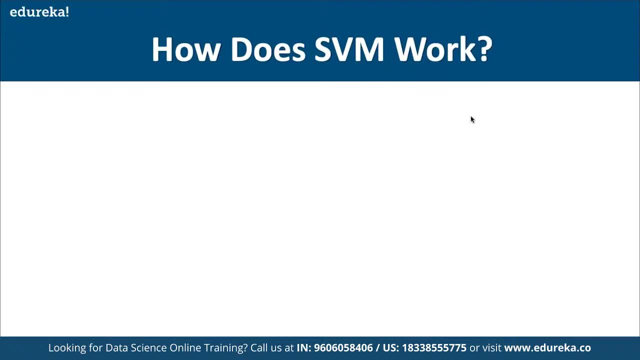 a support vector machine. we can use the support vector machine to segregate the data in the best possible way, and when the segregation is done, the distance between nearest point is known as the margin and the approach is set to a hyper- basically hyper- plane with the maximum possible margin. 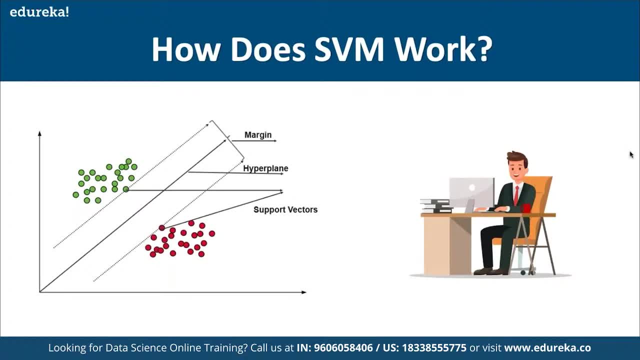 in the support vector, as we can see here. that has been presented. all right and now basically here to select the maximum hyper plane. so now here, in the given sets, the support vector machine follows again multiple sets, for example- is simply going to generate the hyper plane which segregates the classic classes in the best. 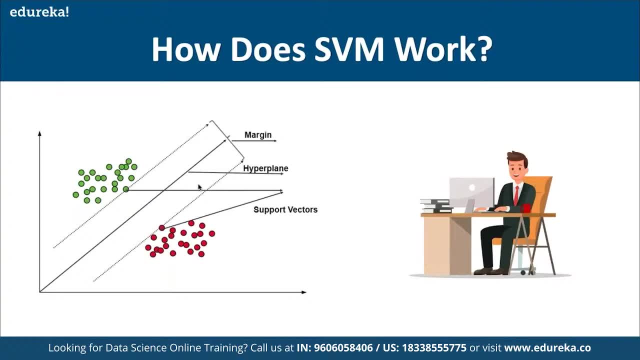 possible way and then we are going to select the right hyper plane with the maximum segregation from either nearest data pointers. so basically, there are different ways of or even dealing with this, and we can see that, for example, we can select a variable or we can say non-linear planes as well. 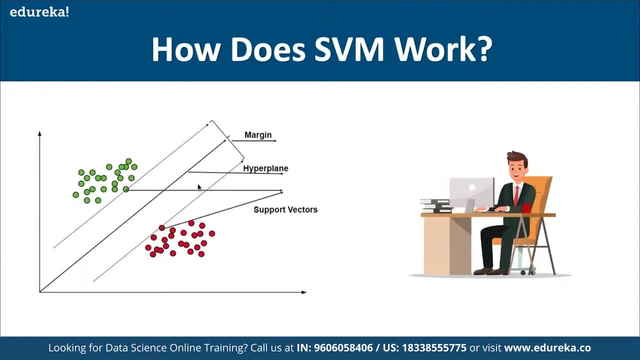 so, for example, in some cases hyper planes cannot be very efficient, and in those cases the support vector machine uses a kernel tick from a kernel trick to transform the input into a higher dimensional space, and with this it becomes easier to segregate the pointers. so now let's talk about 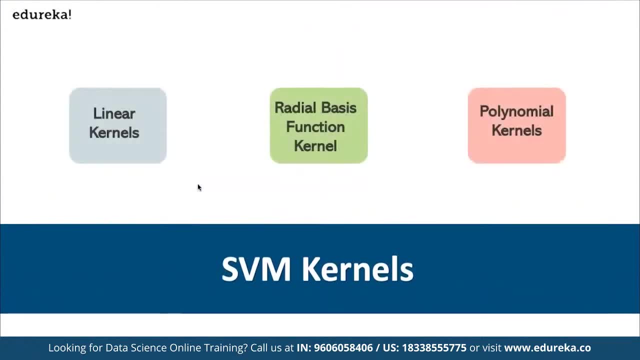 the svm kernels. so basically, svm kernel adds more dimension to a lower dimensional space to make it to segregate the data. it converts the inseparable problem to separate problems by adding more dimensions using the kernel trick and a support vector machine is implemented in practice by a kernel and the kernel trick helps to. 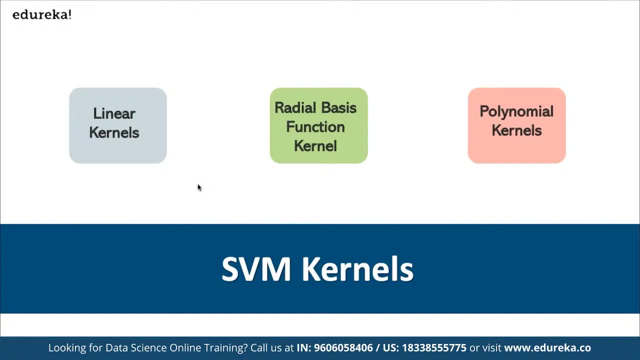 make more accurate classifier so we can take a look at different kernels in a support vector machine, like we have linear, we have radial base and then we have polynomial kernels as well. first of all, let's talk about the linear kernels. so a linear kernel can be used to as a normal dot product between any two given. 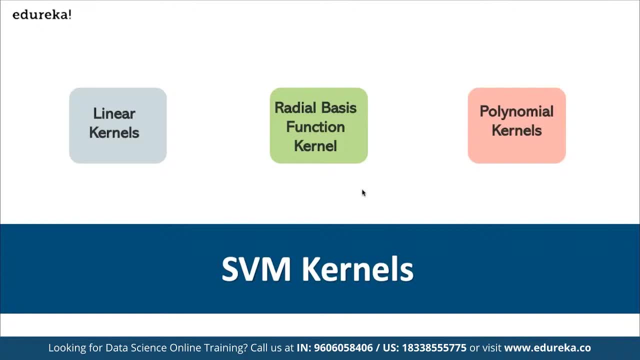 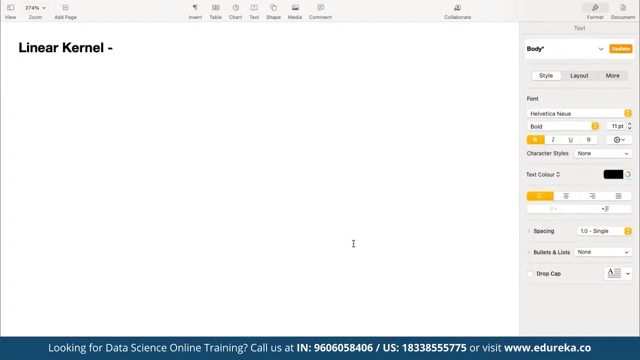 observations. so the product between the two vectors is the sum of multiplication of each pair input values. so we can understand this. so if we talk about the linear kernel, so basically, as we, as we discussed, linear color can be used as normal dot product between any two given observations, for example. here we can: 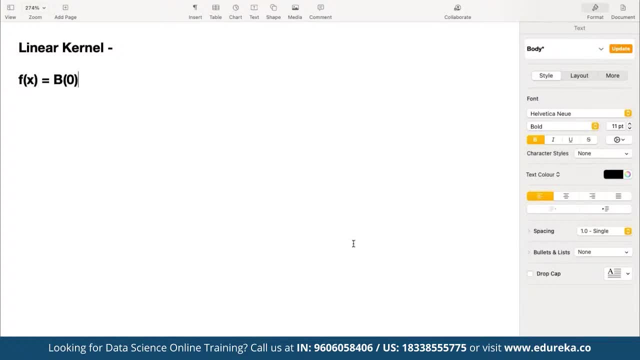 define a linear kernel, and we can define a linear kernel as a normal dot product, and this one, as opposed to zero, and it can be added to sum of, let's suppose, multiplied by X, X, I, all right. so, as we discussed again here, it is going to be: 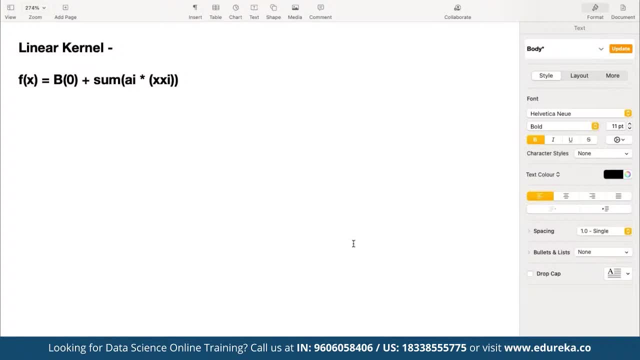 the product between two vectors is the sum of multiplication of each pair of input values as a part of simple linear kernel equation. and then we have polynomial, so this one is for linear kernel. and then we have polynomial, so this one is for linear. then we have for polynomial kernel, so polynomial kernel is for polynomial. 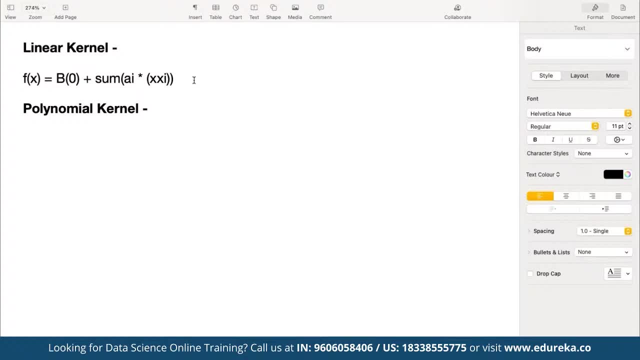 kernel is like, a is rather generalized form of the linear control, and again it can distinguish curved or nonlinear input space. so for example, here we can refer this as opposed as K, and then we can define multiple pointers, I suppose X, 1, X, 2, and then we can simply add this to: 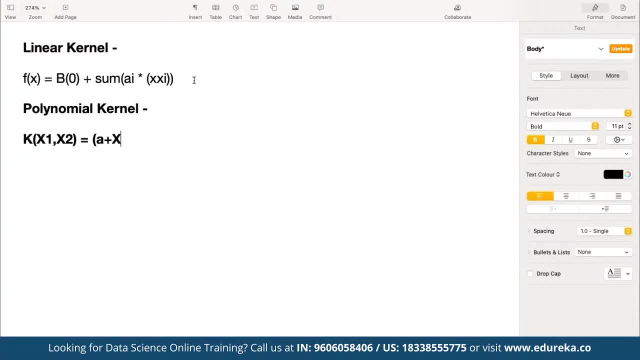 a. now here we have to find, suppose, X 1, and again all of the clicker bit, find here X 1, T, and then X 1, for again it is a value for X 2, here for X 2, and again the entire one has to be raised to. 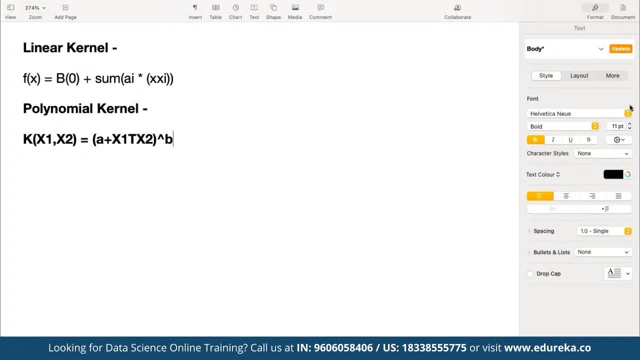 power beats. so next we know, after polynomial we are going to have we also have radius space. for here, after polynomial we have the radial is a function kernel. so in terms of the radius function kernel, so here the radial basis function kernel is commonly using the SVM classification and it can map the space in Infinite dimensions. 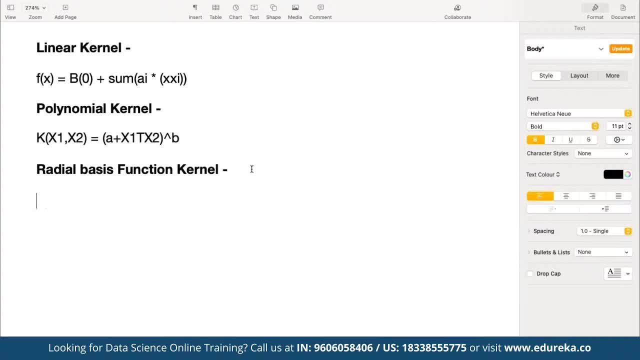 So basically, if we talk about the actual dimensions here, so here we can represent it as opposed the value of K X 1, and again four X X 2, and here we can find the exponent where expert is going to be supposed for minus 4 again become a value and say we represent this as Y, and then we get to 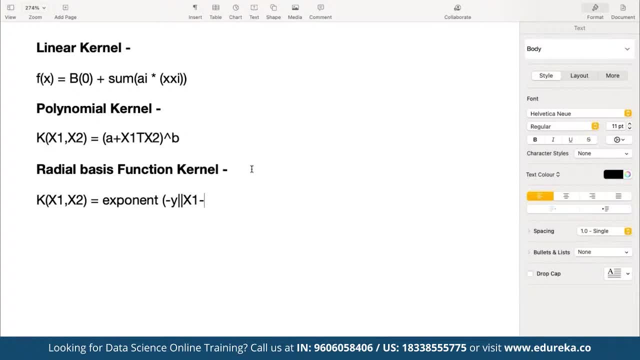 find this for X 1 minus, this is going to be X 2, and then it has to be raised to power 2. so basically, X 1 minus X 2 is simply going to be the Euclidean distance between the X 1 and X 2. so we can say X 1 minus X 2 is Euclidean. 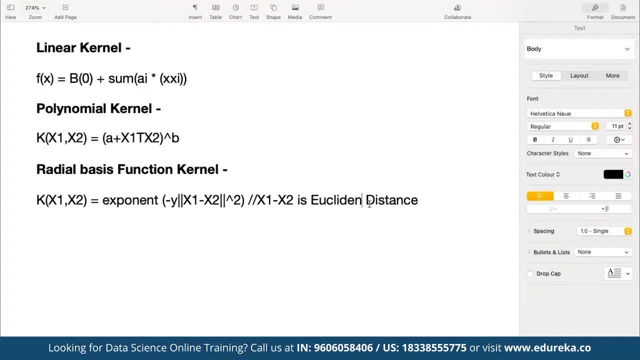 distance is the Euclidean distance between X 1 and X 2. here, and we, if we talk about here, if we talk about the current component for B, so here we can say: B is what B is, B is the degree of kernel. in case you don't have, in case you don't: 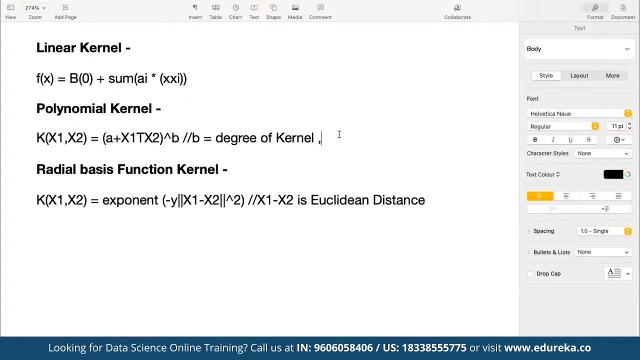 have the knowledge of, of it yet, and then A is going to be. or you can say: A is what is the constant, is the constant term that we have. so here we have linear polynomial and then we have radial basis function, so there are multiple use cases. so, before we proceed further, so there are multiple use cases, all the 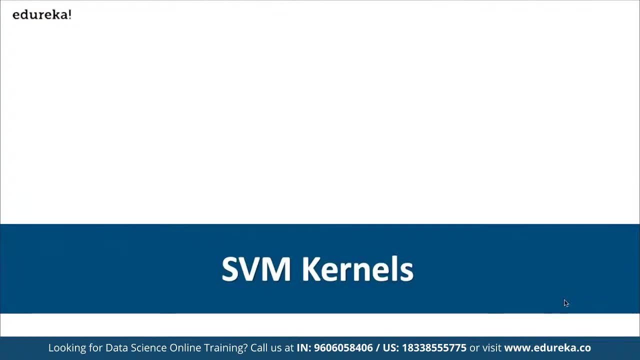 serial base, conver, I can say component as well. so here we can use it for the phase selection for text and hypertext categorization. here we use it for the classification of images, for bioinformatics, for protein fold and remote homology detection as well. we can use it for different use cases and we can also use for again. 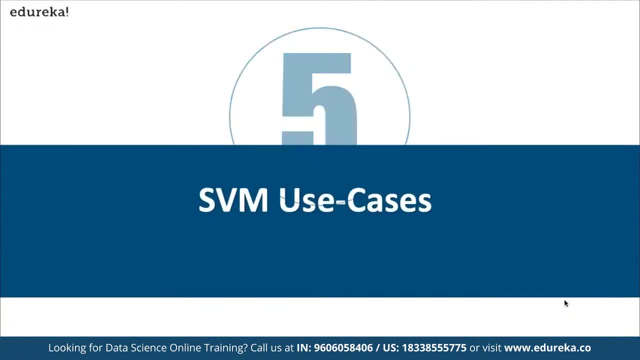 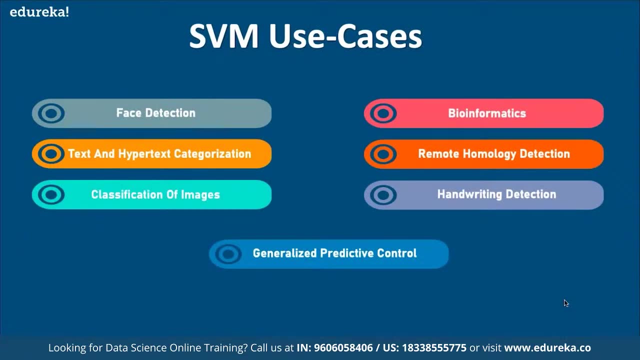 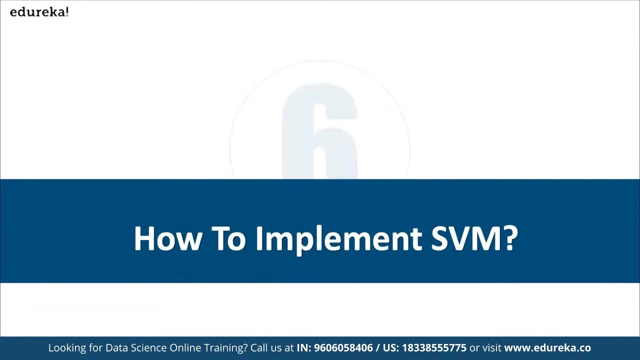 having a prediction control as well, as we discuss in SPM. so there are multiple use cases for phase selection, for bioinformatics, for text and hypertext categorization, for remote hom hating. so these are different use cases currently available here. so now in terms of how to implement SVM. so first of all, 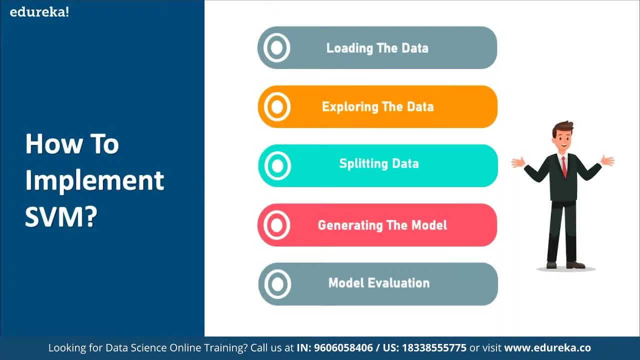 we have to load the data, we have to explore the data, we have to split the data and then we also have to generate the model, and then we have to evaluate the model as well, as we discuss again, in case we have, in computer linear, simply going to be the dot product between the any two given observation奇. 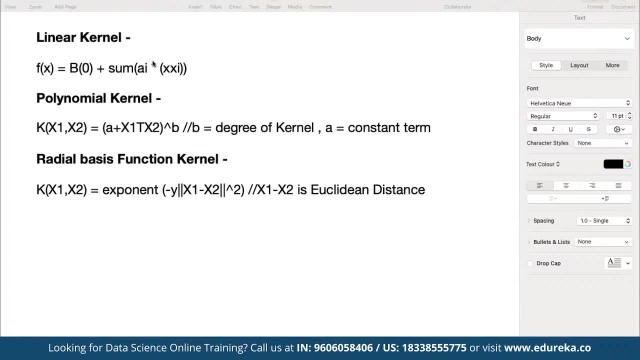 pure dot product between the any two given observation itself, and here we define to. here the product is going to be between two different vectors, it's simply going to be the sum of multiplication of each pair and then under polynomial. so basically here we can distinguish curved or non-linear input space where we have defined 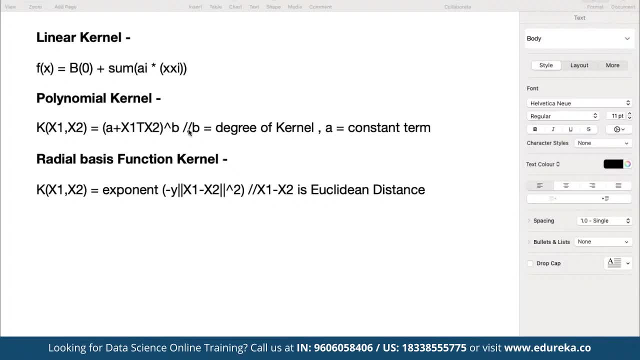 the k1 as x1, x2 for where a is, where a is simply going to be a constant term and b the power to which we have increases. so b is simply going to be the degree of penalty we are going to make use of and then under radial basis, as we discussed. it is commonly used in classification and can map. 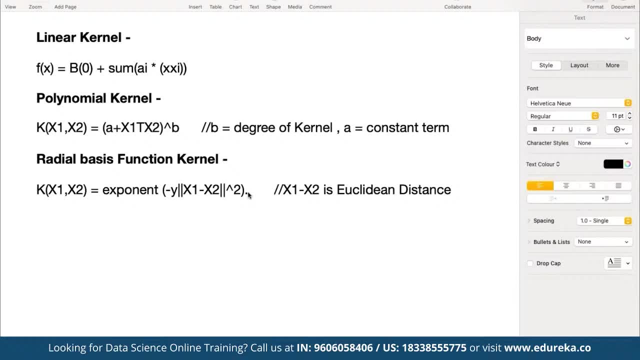 the space in infinite dimensions as well, where x1 minus x2 is simply going to be the euclidean distance sensor, and we can say this one that we define here: x1 minus x2 here is simply going to be the euclidean distance here. all right, so let's do one thing. let's open up pycharm community here. 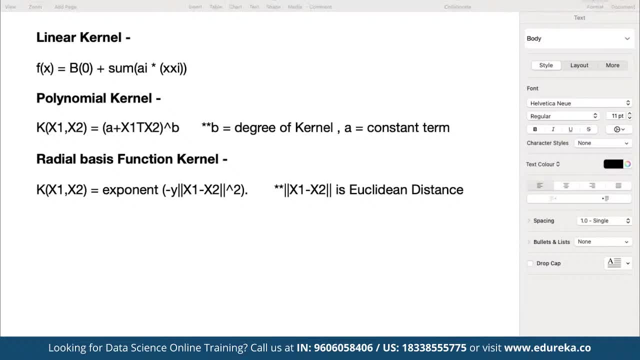 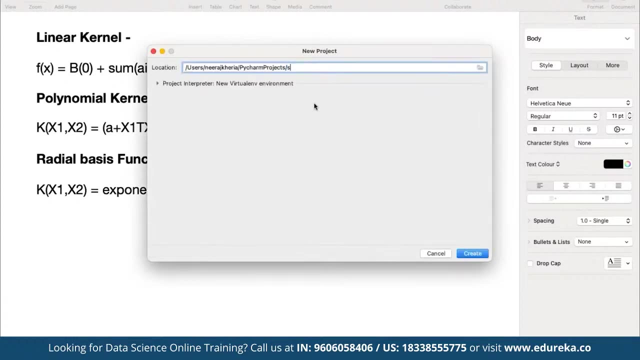 so we can start by simply loading the data set and then working on top of it. so we can use any id. we can use any python id to get started. we can use anything. so let's do one thing. let's create a new project. let's say we name it as svm. 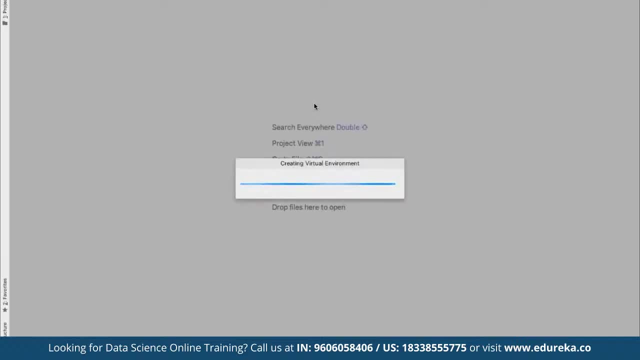 so, in case you don't have the access to svm as of now, so you can go and download the community version. so this is going to give you the access to pycharm, or, or we can use any other id as well, if all right. so here, once we end the project here, we can simply go ahead and 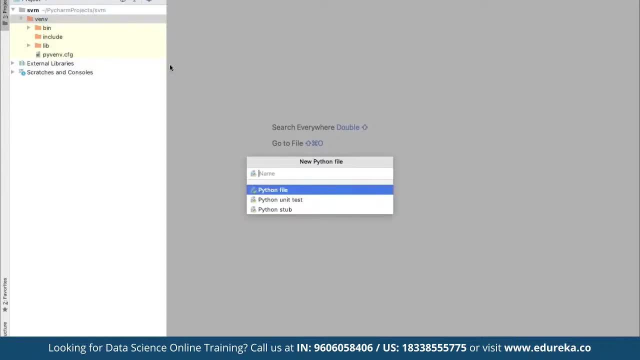 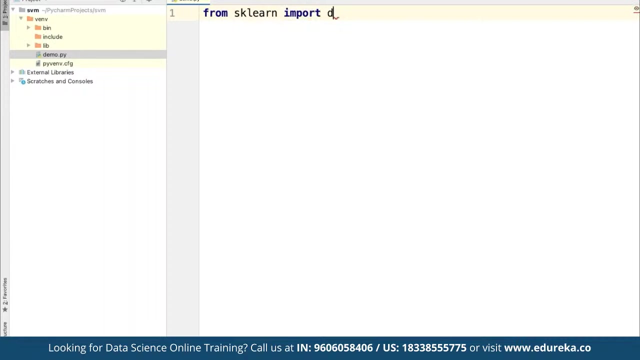 create a new file altogether, so let's name it as our demo file. so first of all, we are going to work from the skln library, so here we can use from skln. we are going to import the data set, so they they are some sample data set available under skln library itself. 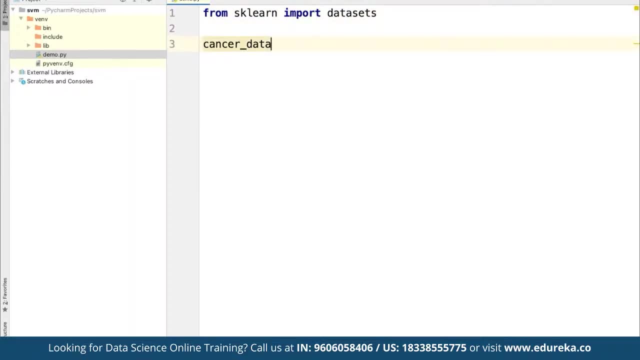 so here we can define the data set we are going to use from the skln library. so here we can define the cancer data set already available under skln and here we can use data sets. start load and then we are simply going to load support for breast cancer. 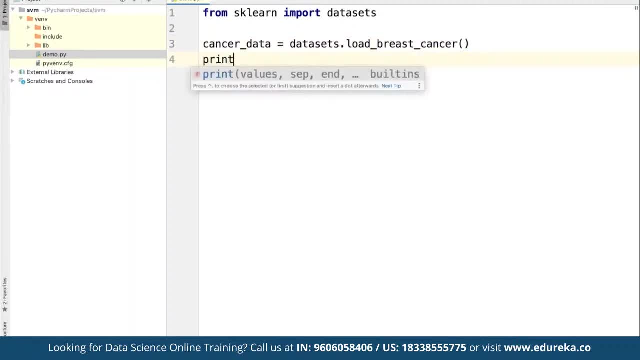 we can load this current data set already available. and now, if we want to simply print the current data set that we have currently imported, so here we can find cancer data, dot data, and again we only want to print the five first rows available in that. so here we can define the statements here. 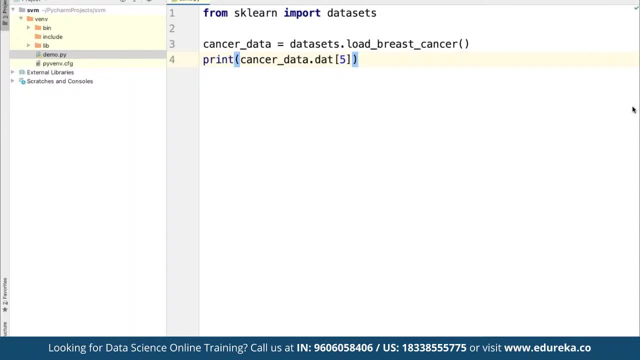 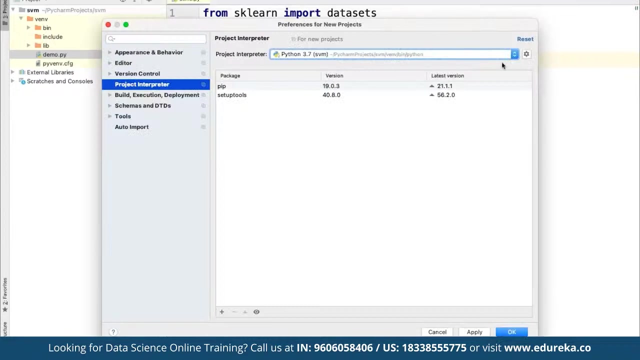 We are going to use a sample data set currently available and Whenever you are going to work on any project, in case they are Now, in case the data set is not available, Then we can go ahead and simply install more libraries by simply choosing the current data set. 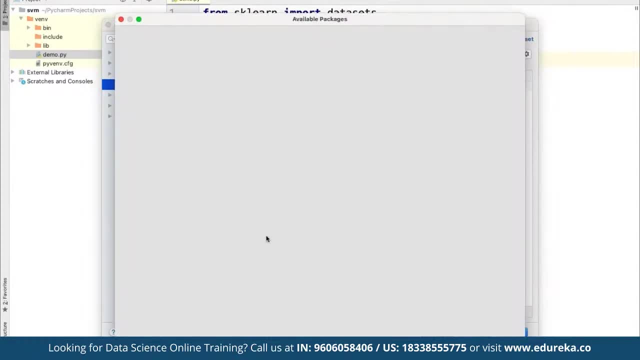 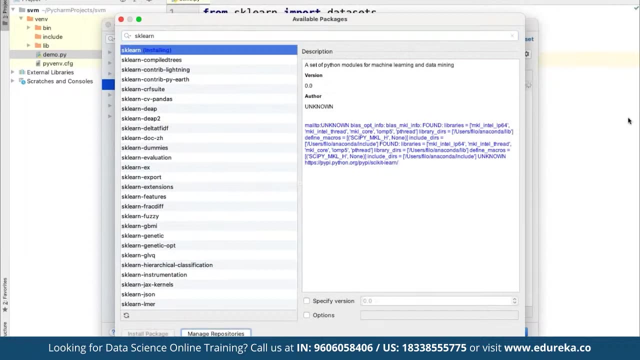 And then here we can go ahead and click on add and from here We can search for any library that is let me me that may be missing. for example, here We are going to work on a skillet, So we have to make sure we do import a skillet, because without a skill library 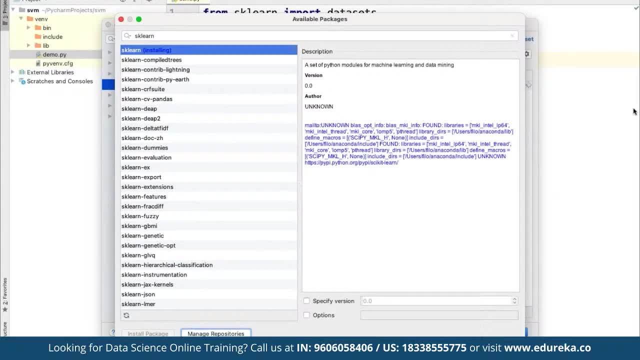 We will not be able to work on the SPM here, So here we are simply going to work on the sample data set. All right, So, as you can see here, now a skillet has been installed. So again, this is a. this is a packet that we're going to work with. 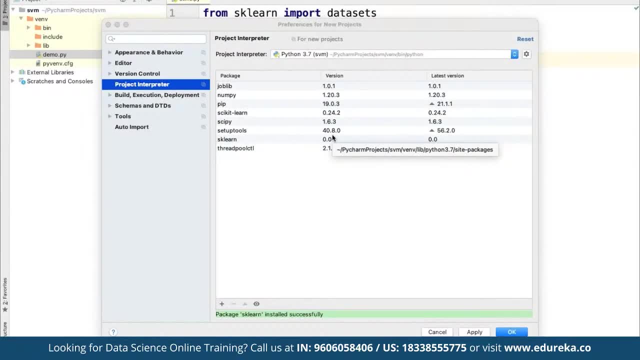 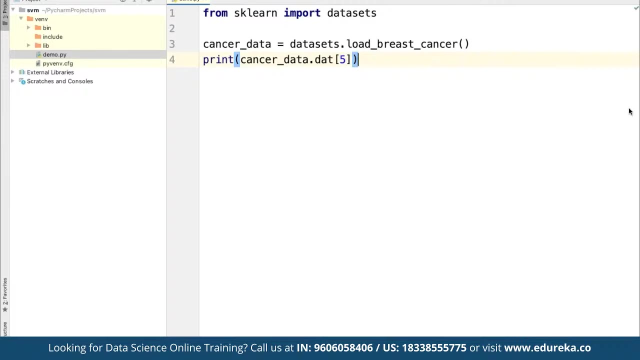 So here we can close it. if we want to work on the other components, We can search for any library and then we can have it installed. All right, so Now we can click on apply and Then, once we top, because if, if we don't have the library installed, and then if we try to run this up, 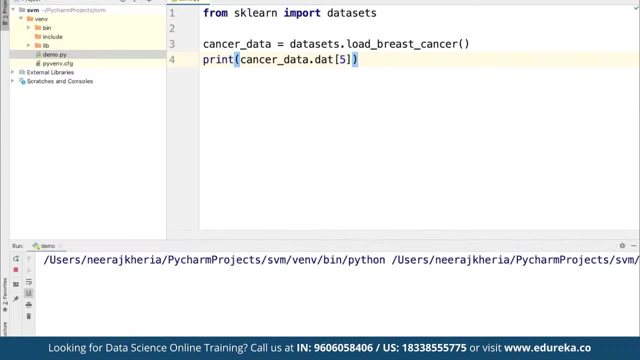 We. it was simply going to throw us an error And, as you can see, currently this is going to update the package and then from there, It is simply going to load the breast cancer data set, which is available as an inbuilt sample in SQL. So it is simply going to get connected to the server and then from there, it is going to be going to pull. 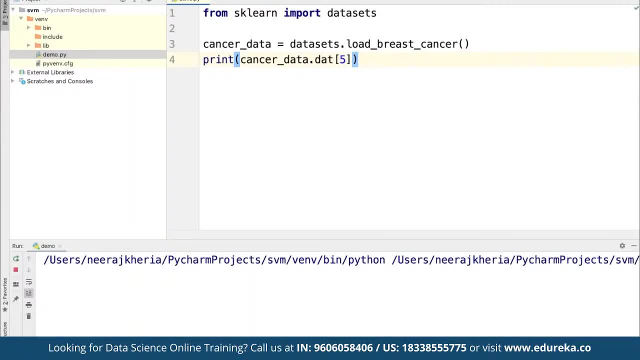 The load the breast cancer leader said, and then it is simply go to print the first five rows from that data set. So it may take a while, depending upon how which there is that we have imported. So before we perform any calculation, let me just show you how static this looks like. 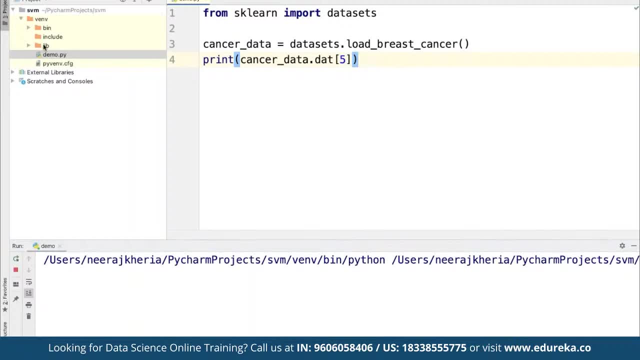 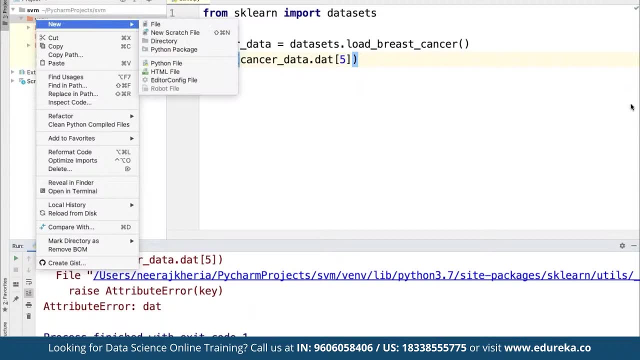 Again in the meantime, this is getting full here, so we can simply go ahead and Create a new file. It has been timed out Because of memory error. Okay, we defined in, Mr Deidre. it has to be detect, certain only. it is simply going to. 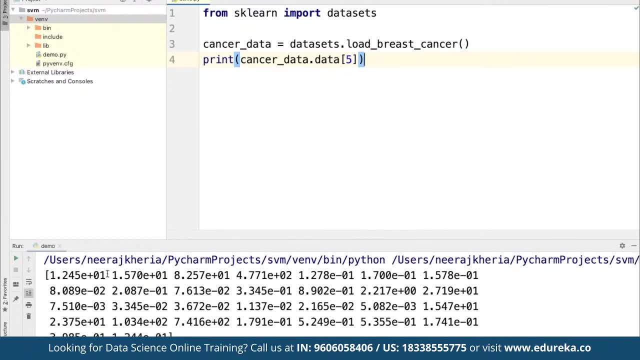 There and Stir hommes again here. now we have the folks five rows in terms of this breast cancer Data, which has important automatically from skm, as against here, right. So now we are going to here, we have defined the dataset right. so no, if we are going to simply. 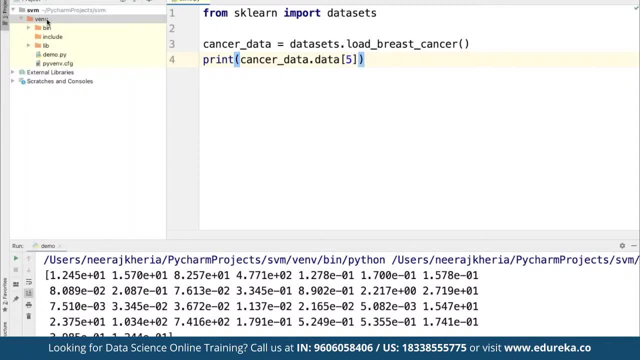 We split the data right. So we are simply going to divide the data into training set and the test set to get accurate results, and after this we will split the data using the train test split function. So here we are going to need three parameters. 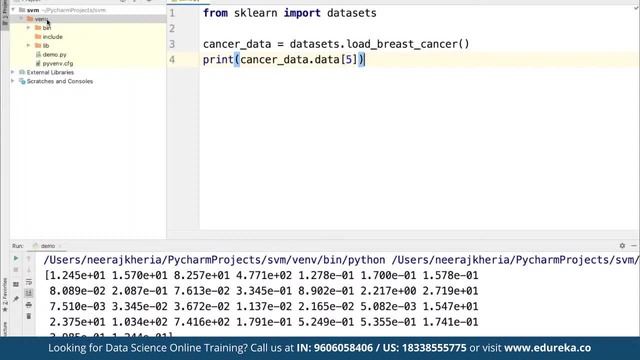 like in the sample that we have that we are going to see. so from here we are going to load the current data set. So for example, now, here, now, just to avoid confusion for your, so we can create a new file, Let's say we define some as supposed to Emma too. 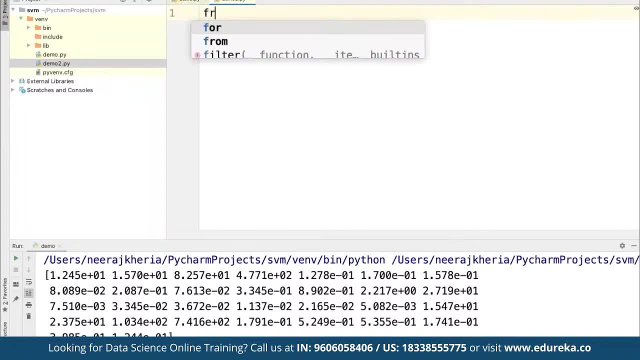 So here we can find from sklearn. So first of all we define from sklearn library, from sklearnmodel, and here we can define model selection. So here we are going to import train test split, as we discussed, We are going to split it, and then we can define from cancer data. 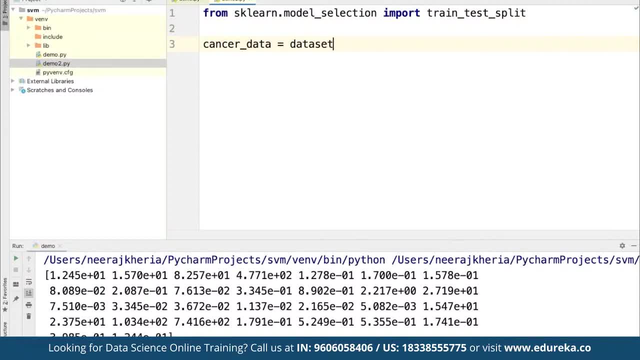 that we are going to import. So here we are going to find data set, dot load, Rest cancer, which is already available, and then we are simply going to define the models in terms of: suppose, here we define extreme, And then we can find X split, we get a plan for X test. 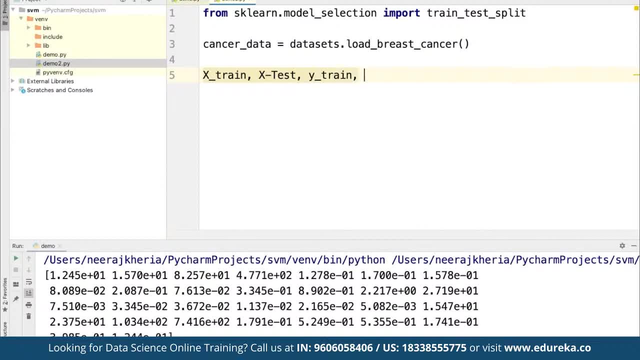 and then we get a fine same thing for Y train, For Y test, X train, X test, Y train, Y test. So here we are going to define this from the same train test split that we have going to import, and then here we are going to divide. 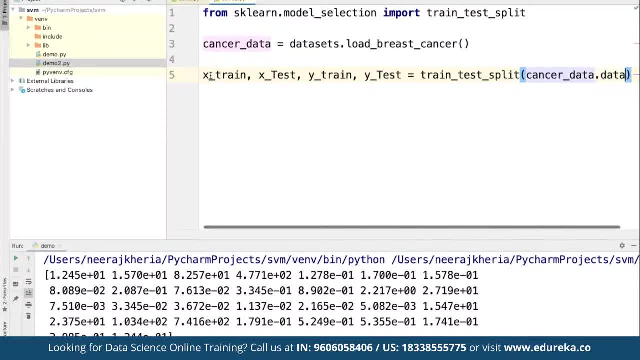 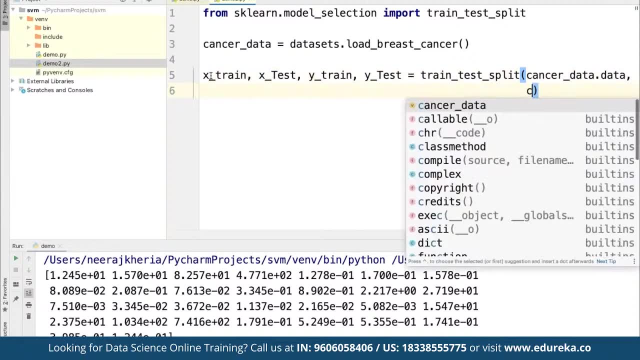 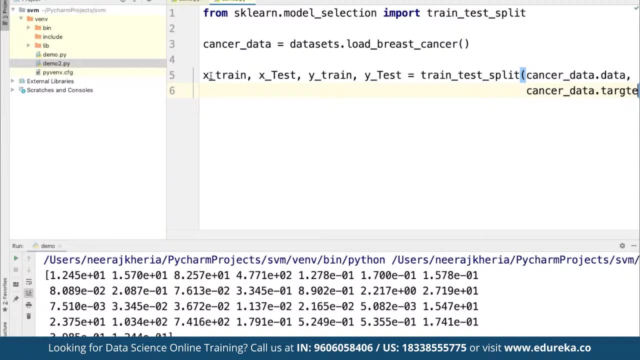 them under from the cancer data and the data which has been imported here, and then we are going to define this for cancer data target. So say, here we can find this for cancer, So here we can find this for cancer data target, And then we can find the test size here. 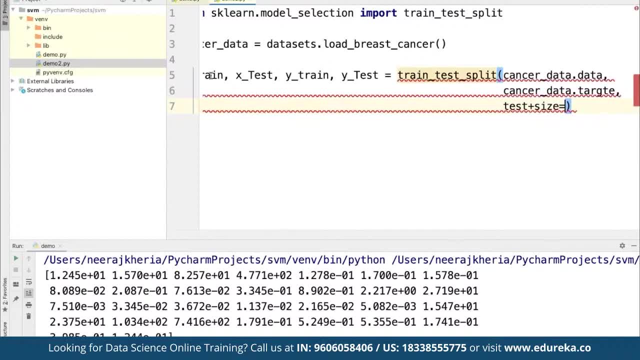 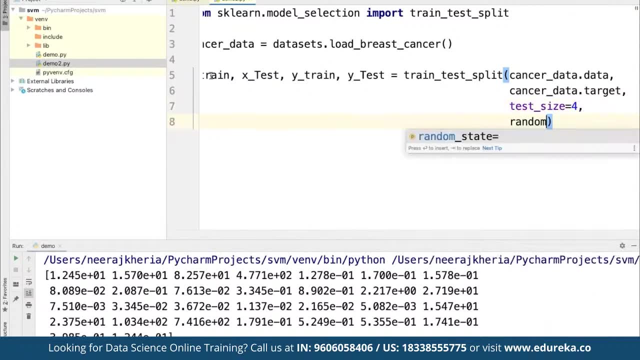 We get to find the test size. Suppose we want to keep the test size opposed as for. this test has as for, and then we're going to find random state. We can find random state as opposed, But I don't like anything that you want to have. 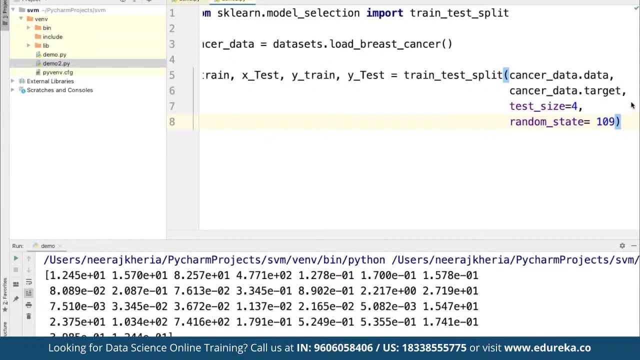 So here we are simply going to split the data set with the given in the X train, X X test and the Y train and Y test here. So here the entire set is going to be going to be split. So, as you can see, now that we have split the entire data set, 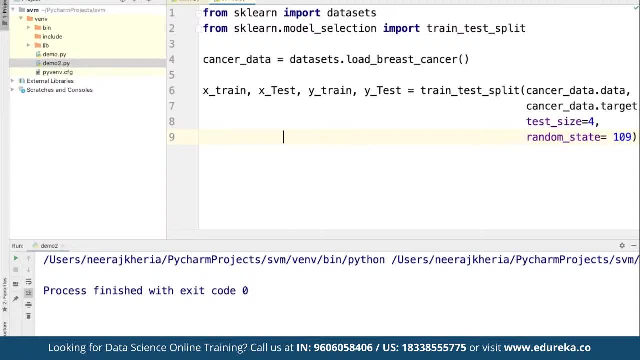 So now we are going to generate the model as well. So what we can do. So now, here we are going to change. we can say: generate the bottle and for that we can import. on the library, For example. here we can import, let's say, a scalar. 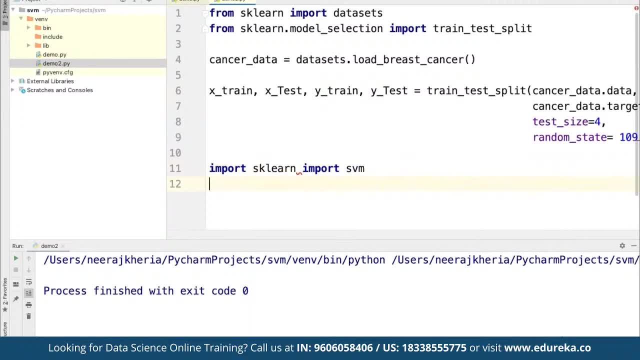 and from escalon We are going to import the SVM, So here we are going to create the library, So here we could create a classifier here. So first of all we're going to find classifier as opposed SVM, dot, SVC, and here we can find the kernel here. 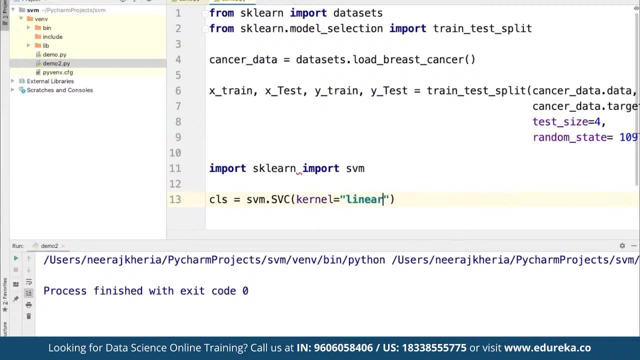 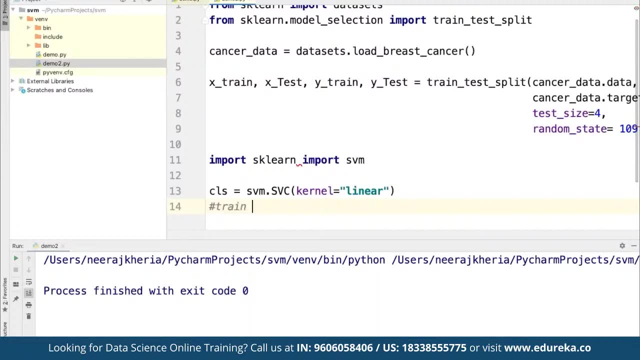 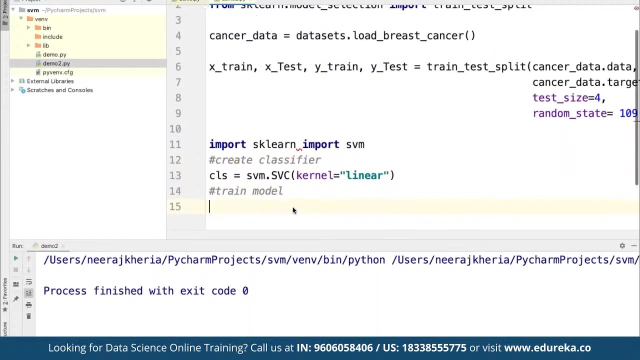 We can find the kernel, as opposed linear. whatever we want to use, We can find that and then we are going to train the model. so you can see, we are simply going to not train model. So here we have create classifier And now we are going to train the model. support green the one. 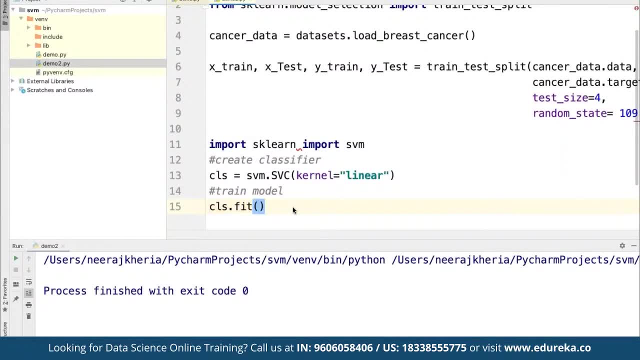 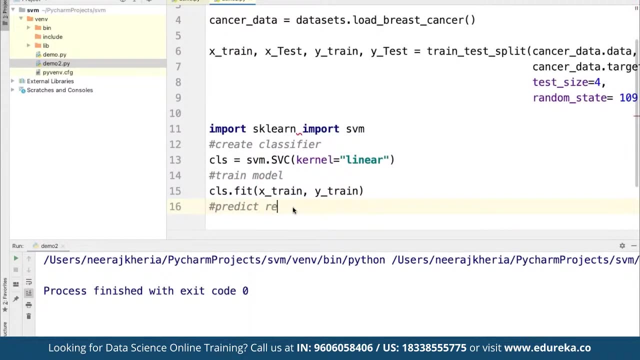 we can define class, dot, fit, and then we can define this value as extreme that we have already imported, and then we can define for Y train that have we have already performed the split on, and then simply we are going to have a prediction done. So here we can define predict response and for getting the response 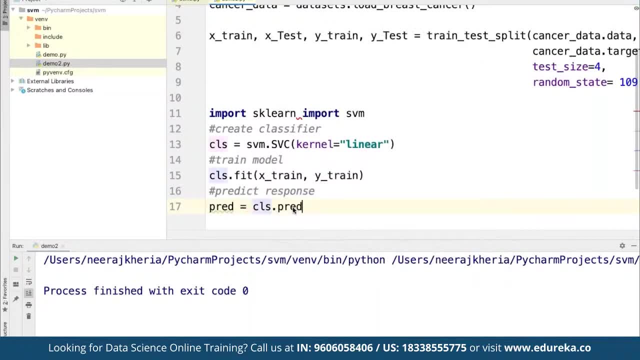 we can define prediction as class dot predict. for this we are going to make use of X test that we have already defined. we had to find for extreme and for Y train and then for prediction. We are simply going to do that on the text on the X underscore test. 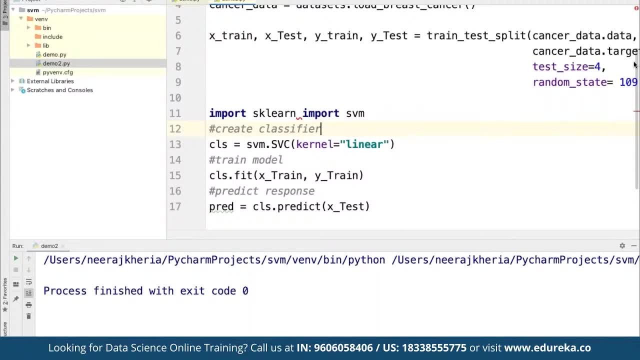 is that we already have to find that depends upon type of data that we have. So that totally depends upon the type of data We are going to simply import and let's move this import from the end up here. So you have to find this. 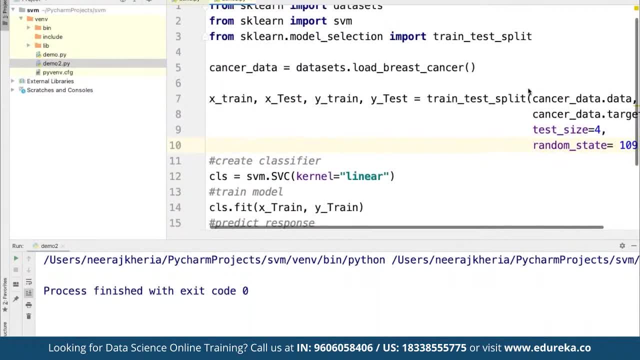 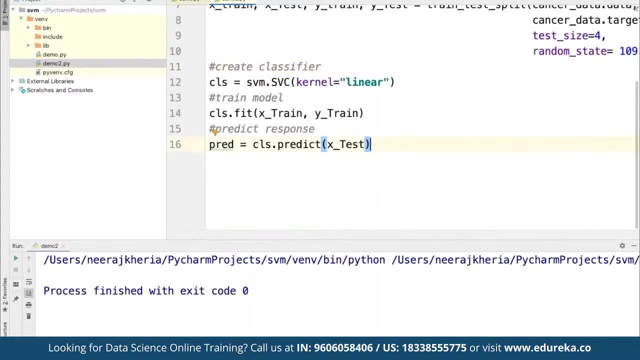 the top section is up from a skill and we are simply going to import the estimate we had to find on it, and then we had to find a classifier. Now we are going to evaluate the model, and for evaluating the model, we can simply go ahead and define. 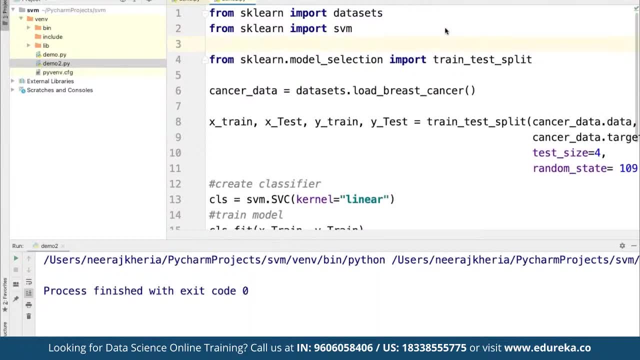 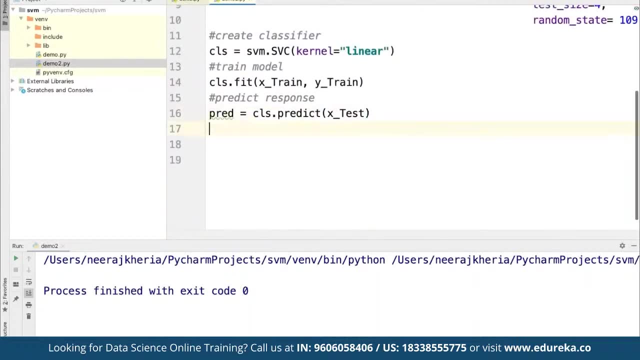 So here from a skiller, we can also import other components as well from a skill and we are also going to import metrics. So here we are also going to import metric and by using back your accuracy metric for getting the accuracy We can find, for getting the accuracy. 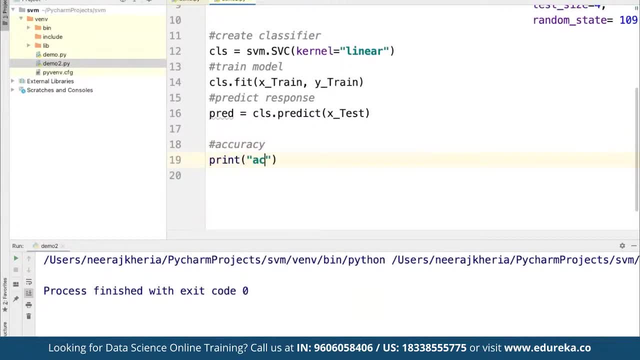 We are going to define. we are simply going to print the accuracy of the prediction here and for accuracy, We are simply going to define metrics, which is again available. under the metrics that we have, We have accuracy score and then from here We are simply going to find why test and we are going to finance before. 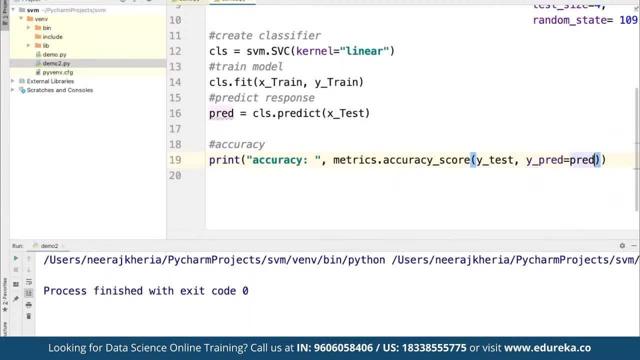 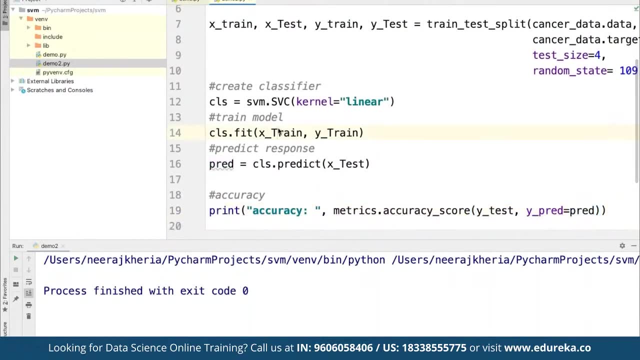 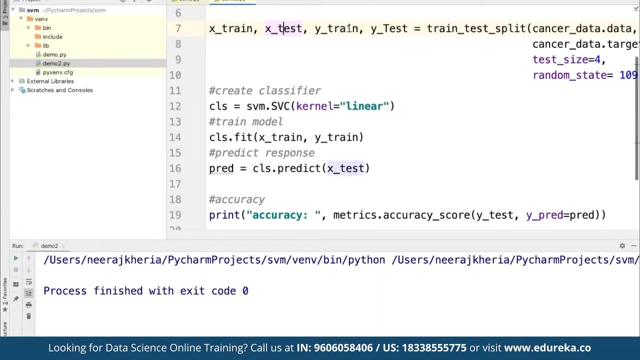 why prediction as well, that we have defined. second, We have used, why test? we have used up our case for, for we have used less. one thing, Let's use small case for everything. just to word confusion. That's a fun, says test, train and test again. 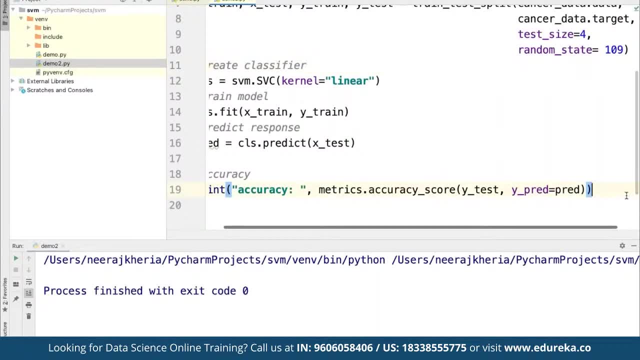 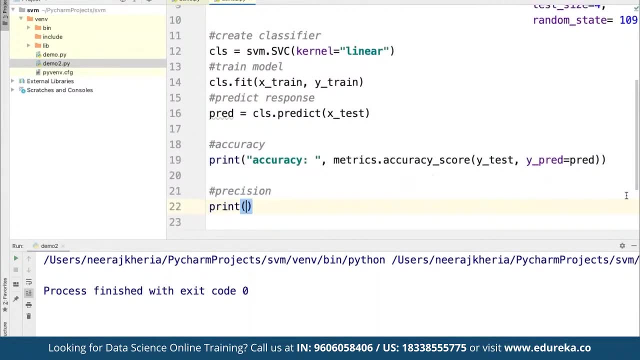 So you have a why test, and then you depend. here We define it for production and then for finding the precision score. for finding precision We can simply print another statement as precision score, And in here we can again make use of metrics, and for metrics we can define the precision. 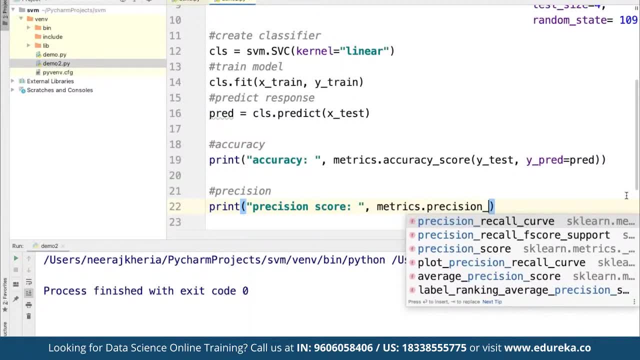 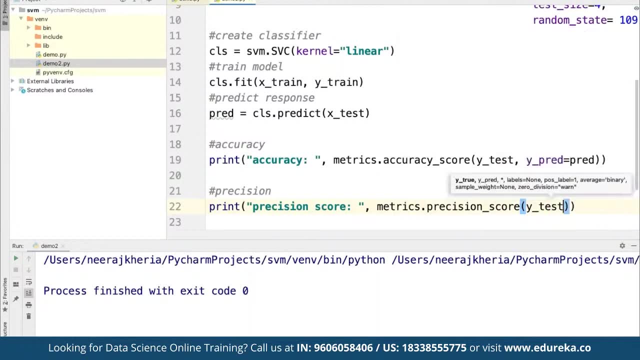 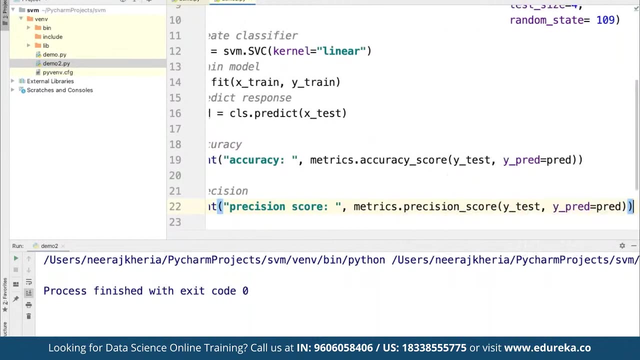 Score itself. So here we can define precision underscore score, and in here, for precision score, We are going to make use of y test, and then we are going to make use of y prediction, All right, and then at the end, if you are simply going to recall the score, 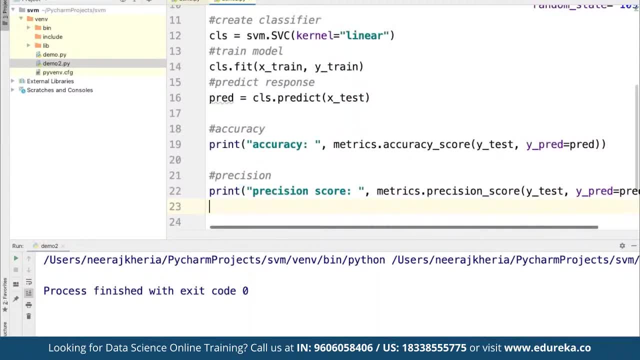 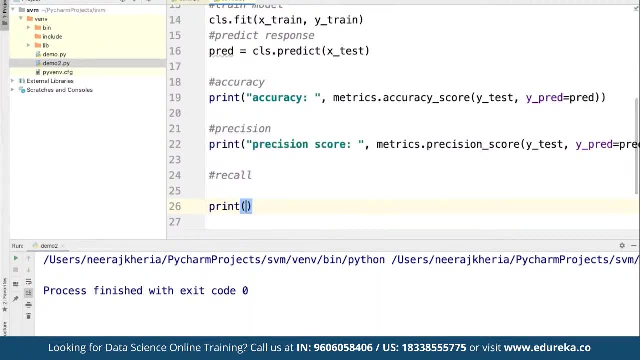 and we are simply going to put so here we can find for recall We can print another statement For recall, we can define this one as recall and here from save metrics, dot recall Score, and for here we can find why test and why prediction. 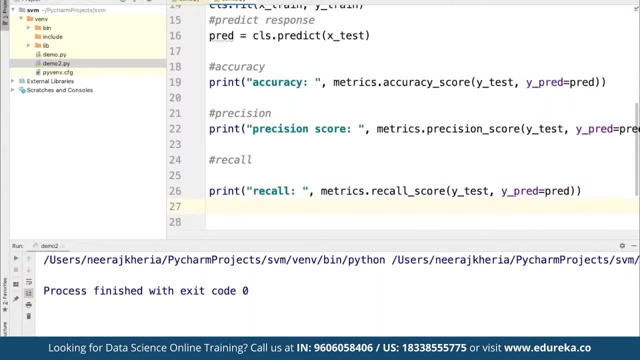 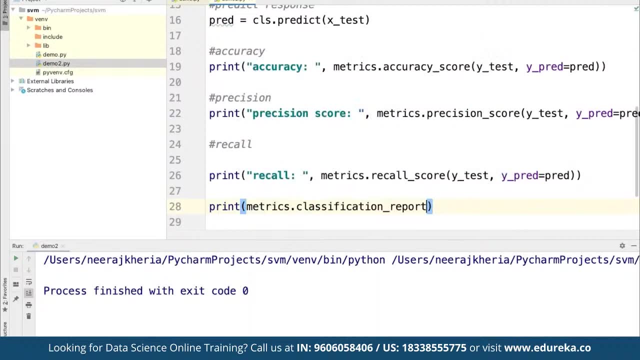 for the prediction that we are going to define. And then, if you want to print all the metrics, so here we can find print metrics, dot classification report and for that we are going to make use of y test. And why? Prediction for prediction made. 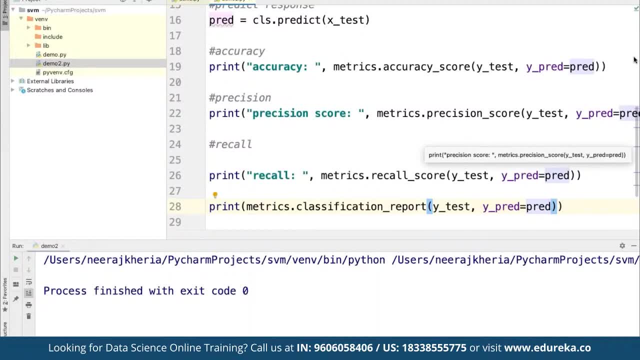 All right. So here we had to find these, and now, once we have configured everything, So here we can simply run this up and we would be able to see the entire output which, once it has been defined, So now we can see. here We have the accuracy here. 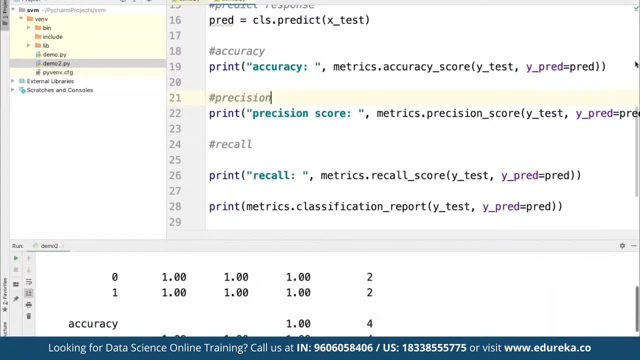 We have the precision score, the recall score that we had to find, and then we define the accuracy based on whatever data we are going to work on. depending upon that, We are simply define the current data set here. Thank you so much for joining, guys, and have a great day.